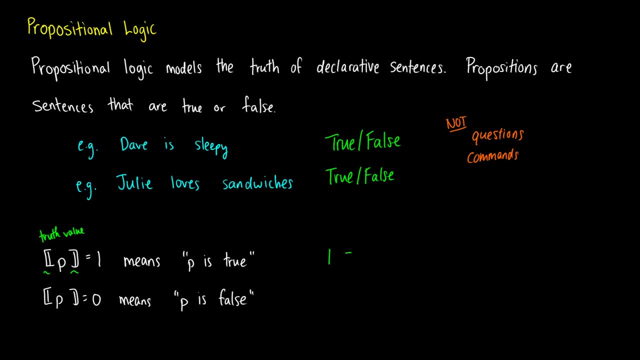 of P equals one means that P is true. So if you ever see one, that means true. And if you say that the truth value of P is zero, that means that P is false. So zero is equal to false. You may see these written in books as T's and F's. Sometimes they're stylized. 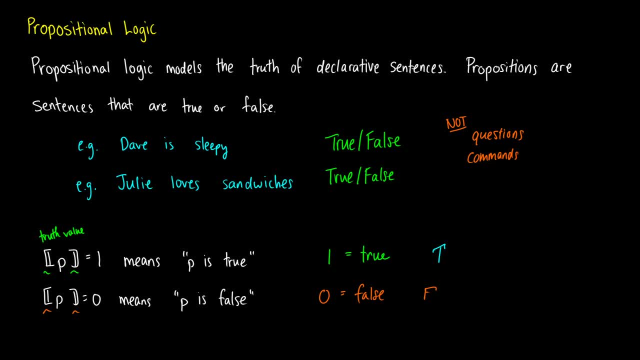 sometimes they're not, But it's actually everywhere outside of intro textbooks. in philosophy we use ones and zeros, So that's just a convention to get used to. Now we can take simple propositions and we can combine them into more complex propositions, which are called well-formed. 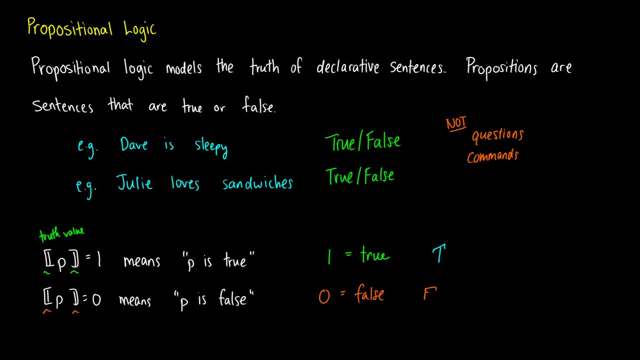 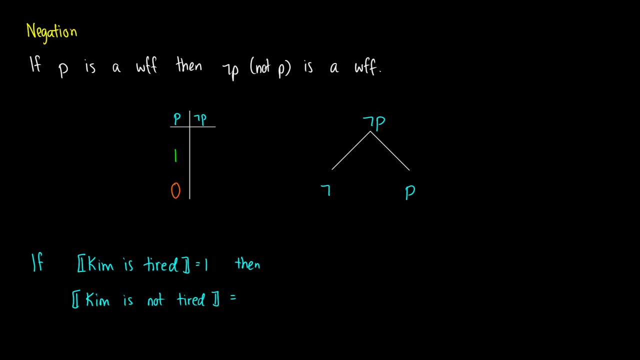 formulas or WFFs woofs. So the rest of this will be basically going through all of those different operators and taking a look at how they combine with their truth values. So negation is our first one. this takes a single proposition and it negates it. So this: 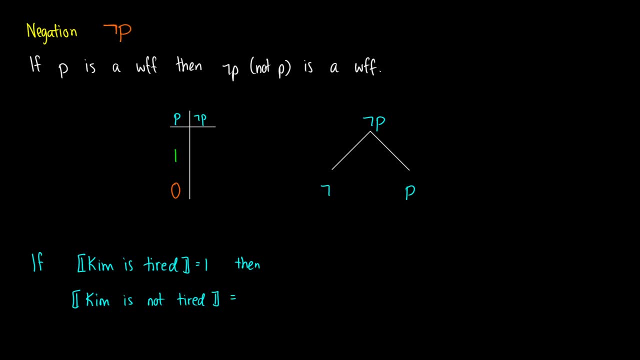 is when you have a proposition P, you can make a proposition not P. So we have this little bar that means not. So if P is a well-formed formula, then not P is a well-formed formula. What you're seeing on the left here is something called a truth table, And what this does is 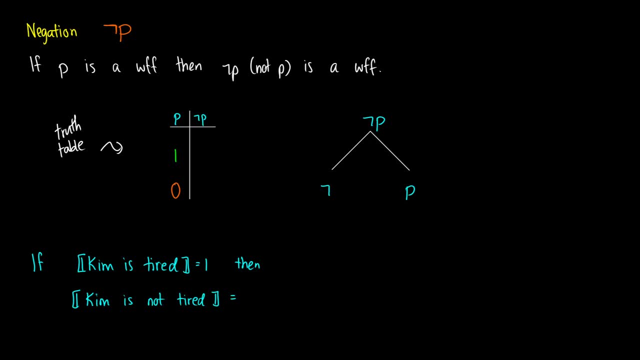 this tracks the truth of things. So it says, well, let's go over here. This is the actual result of the world. The longer this is, the harder it's going to be to get to the truth. So it says what happens if P is true. 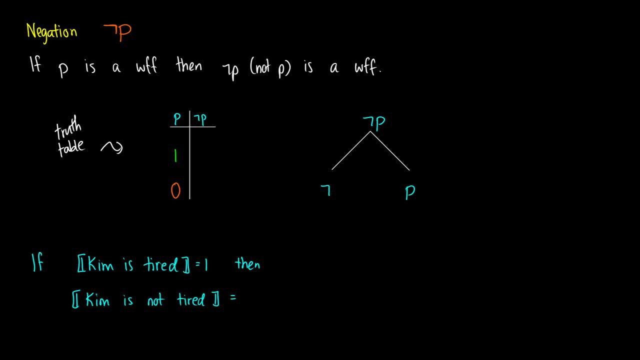 What happens if P is false? What does not P do to the truth value? So what we see is that if P is a true sentence like I am happy, then not P. the sentence I am not happy ends up being false. 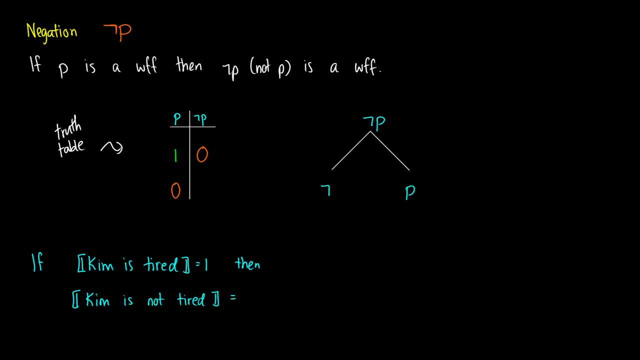 While if P is a false statement like I am happy is not true, then sorry. if P is false, so I am not happy- we're saying I am not happy- is false, then the sentence I am happy, which would be the negation, would be true. 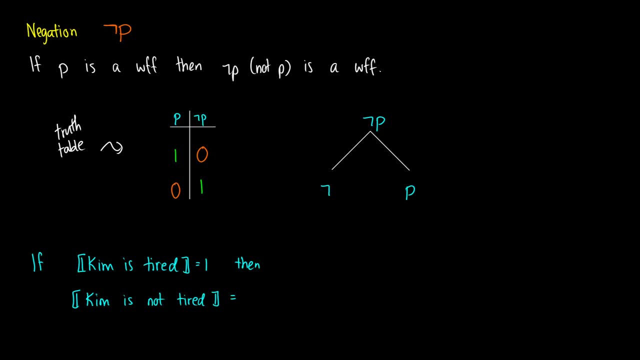 So you can think of not as flipping the truth value of a sentence. So that's what the truth table looks like for not P. On the right, what we see is its syntactic structure. So, in order to build a sentence like not P, 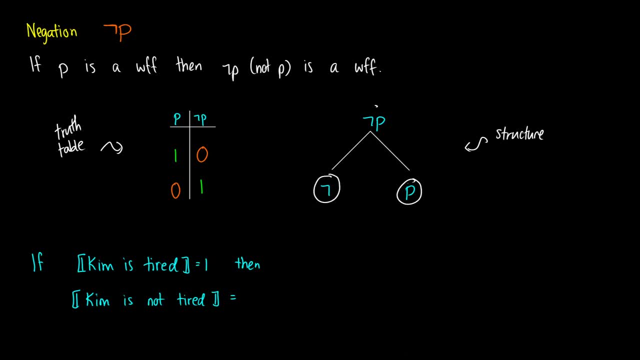 we need to have some proposition P, we need to take the operator and we join those together to get not P. So that's how we use our structure there. It just takes one proposition. Now our bottom is our sentence example. So if we say that if Kim is tired is equal to one, 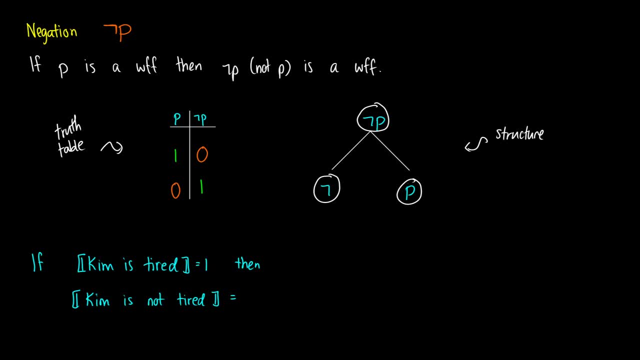 if that sentence is true, then Kim is not tired would be false. So here is our English equivalent of it: not tired. We can do to get these values here. one and zero is. we can take a look at the chart. So if Kim is tired is true, 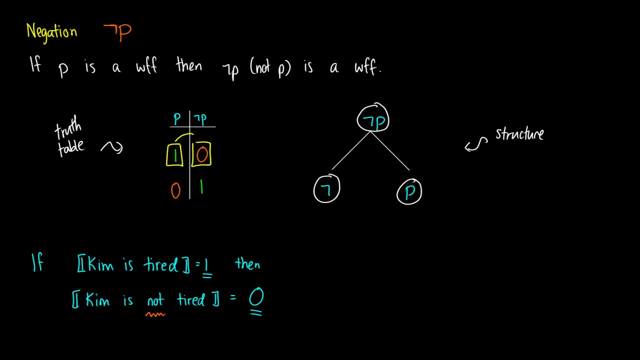 so this is gonna be this first line here. then we know that Kim is not tired is going to be true. So that's flipping the truth value. So this is what you need to know for negation. The second one we'll look at is conjunction. 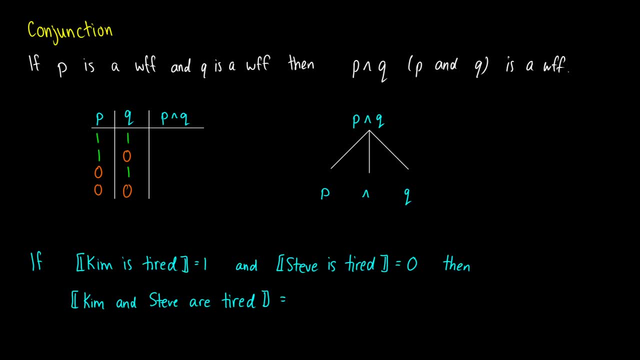 So this requires two well-formed formulas: P and Q. So if P is a woof and Q is a woof, then P and Q. so we write this with like a triangle without a base, meaning P and Q. that's also a well-formed formula. 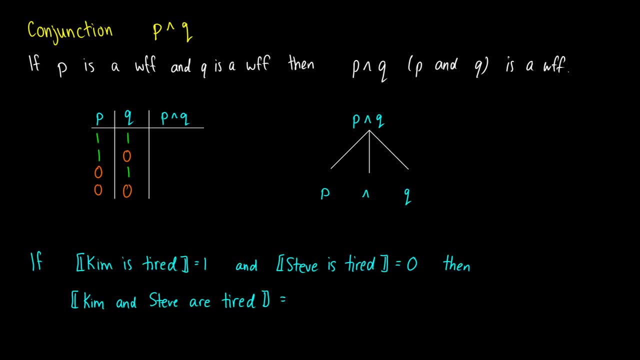 Now what we see in our truth table is four rows instead of two. We need to take a look at the combinations of truth. So when is P true, when is P false, when is Q true, when is Q false? and take all those combinations. 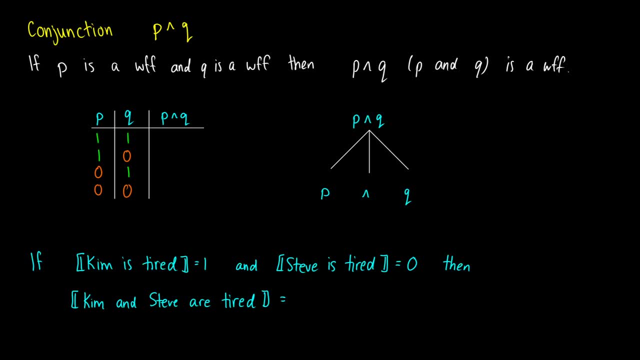 So the way that the conjunction works with P and Q is: it's only going to be true when both P is true and Q is true. In every other case it'll be false. So, if you can imagine, I'm hungry and I want a drink. 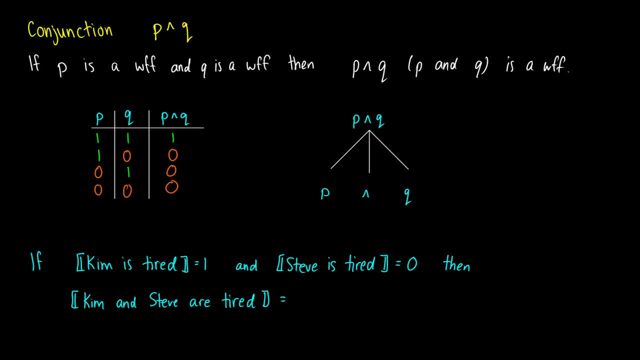 that's only gonna be true if I'm hungry and I want a drink. If I'm not hungry, then the combination's not gonna be true. And if I don't wanna drink, the combination's not gonna be true. That's what the truth table looks like for the conjunction. 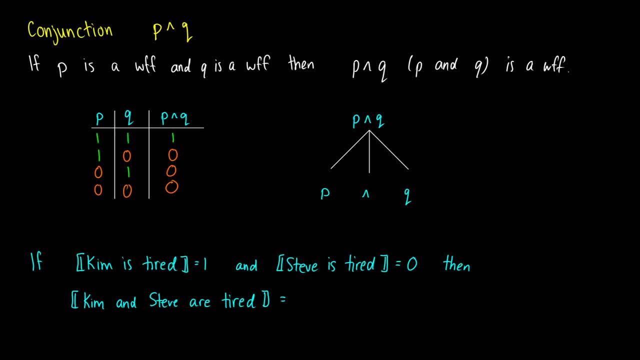 In terms of its structure. this requires two things. It requires a proposition P, a proposition Q, and then we take the conjunction to build up to our P and Q. So this is three branching. it's ternary branching. So with our sentence example, if Kim is tired is true. 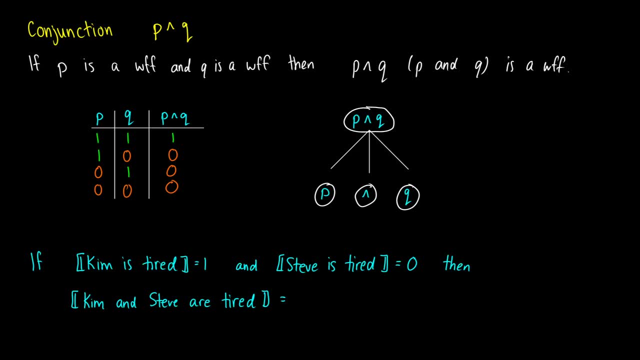 and Steve is tired is false, then the sentence Kim and Steve are tired would end up being false. And we can just take a look here. So we see we have a true sentence, we have a false sentence. So this is looking at line two. 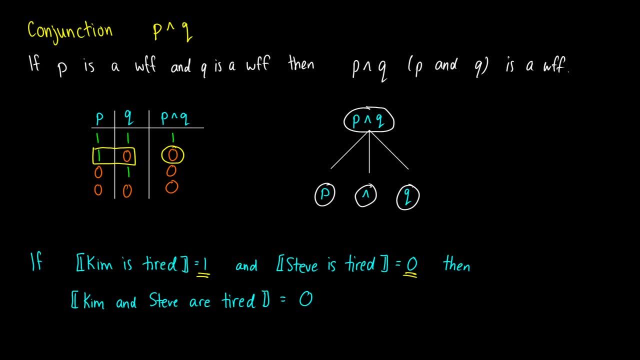 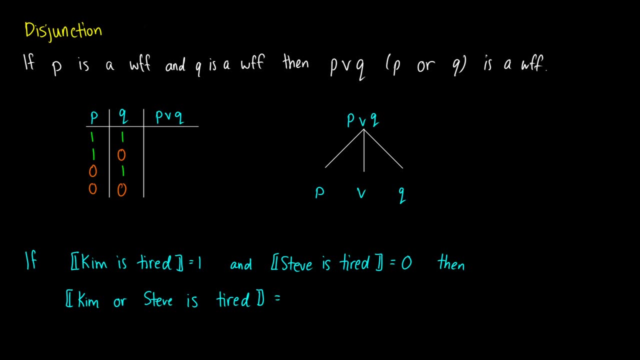 So when we combine them, our result is going to be false. So that's our conjunction. Our disjunction is about the word or. So this is P or Q. we just use a V symbol for this. So if P is a woof and Q is a woof, then P or Q is a woof. 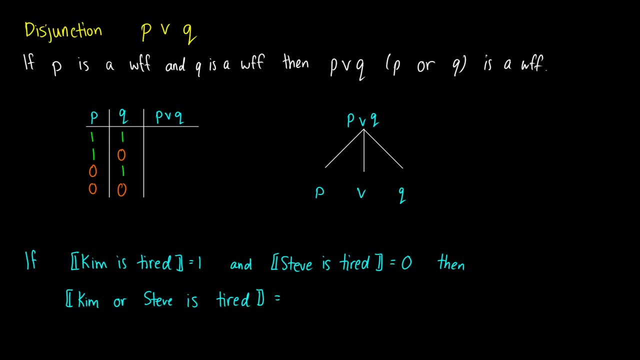 So, in terms of our truth tables, P or Q will be true. if P is true or if Q is true, As long as one of those two statements is true, their complex woof P or Q will be true. So that means in the first three rows it's going to be true. 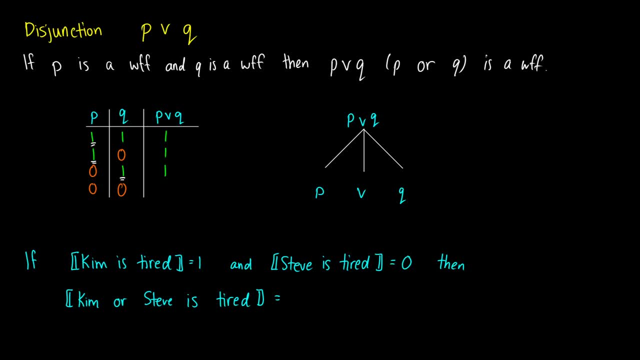 because we have at least one thing being true in each of those rows. But in the case of the fourth row, neither of those disjuncts are true, So P or Q will end up being false. So the structure is very similar to and. 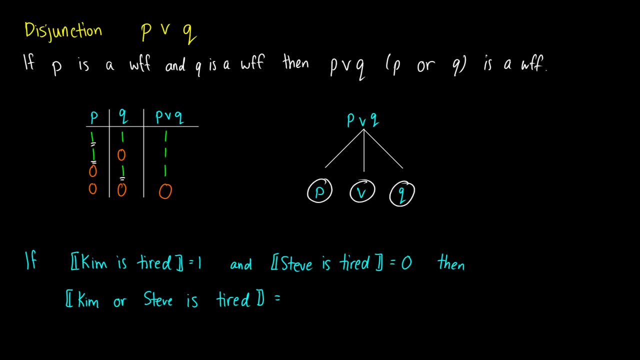 It takes two propositions, P and Q. It combines them with or to get P or Q. So with our sentence example, if Kim is tired is true and Steve is tired is false, then Kim or Steve is tired will end up being true. 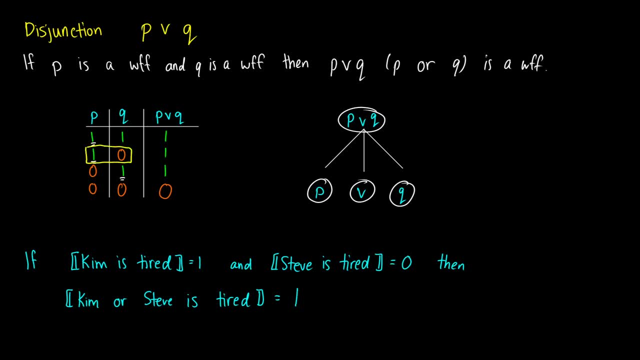 So in this case we're just taking a look at our second row here. At least one of those things is true. Kim is tired. Therefore, the disjunction of them will be true as well: Kim or Steve is tired. The last operation we're going to take a look at. 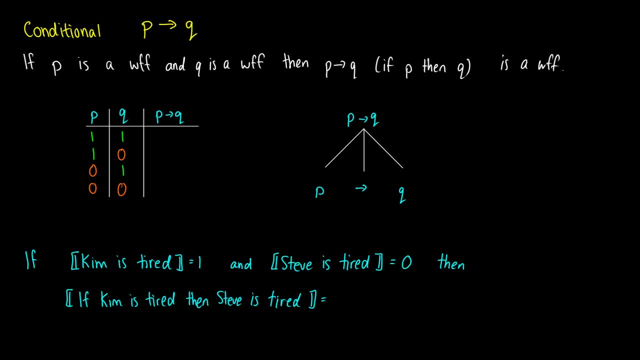 is the conditional. So this is: if P, then Q, So you can think about the arrow as being the word then. So if P is a woof and Q is a woof, we have P arrow- Q is a woof or P, or if P, then Q is a woof. 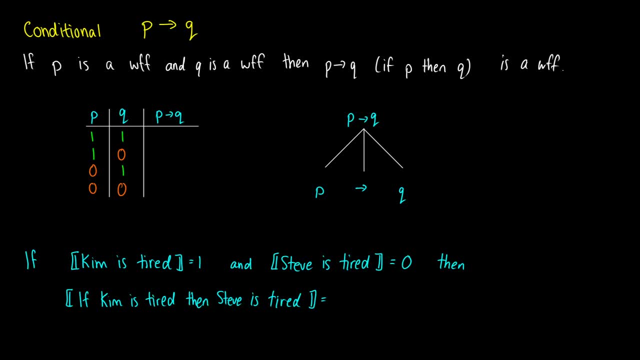 In terms of the truth table. this one's a little bit more interesting. It's going to be true in every case, except for when we get like this lying behavior. So imagine, I say, if you eat dinner, you'll get dessert. 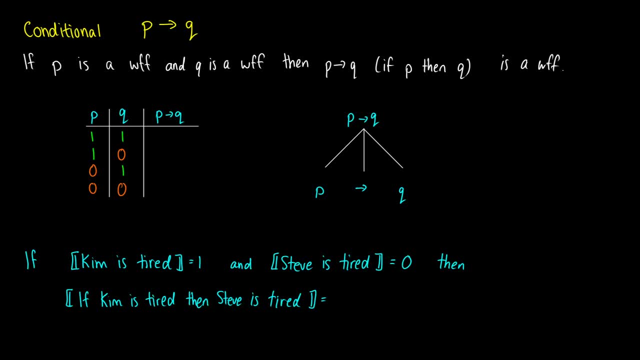 You eat dinner, what do you expect? You expect to get dessert. So if the condition is true, our consequence should be true as well. But in the case of the second line here, 10, that's like saying if you ate your dinner, you get dessert. you ate your dinner, but now i'm saying no. 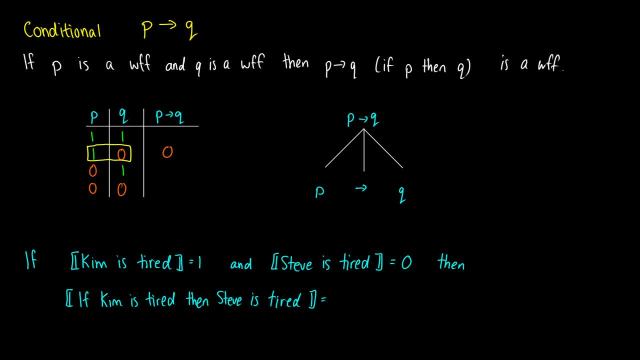 you don't get dessert. so in this case it's going to be false, but every other case is going to be true. so this is what our truth table looks like. our structure is similar to the conjunction and disjunction and, in terms of our sentence example, let's say: kim is tired is true. steve is tired is. 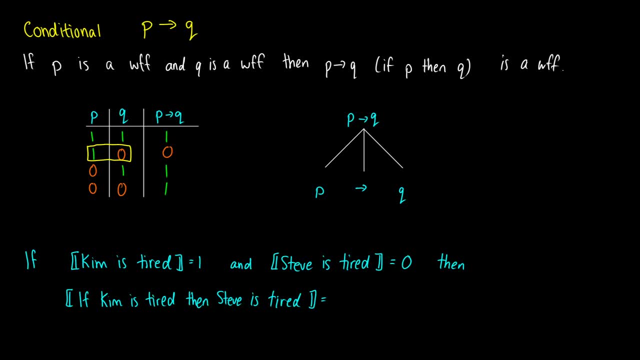 false, just like before. and then we have the sentence: if kim is tired, but then steve is tired. so this is like saying that kim is tired is true and then steve is tired is false. so we have one arrow zero. so our result is also going to be false in this case. now there is a special term that we 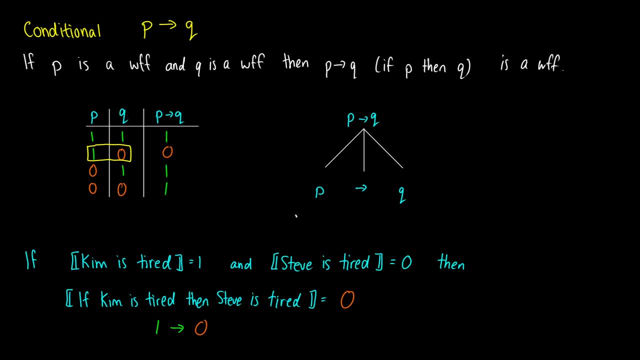 should learn with conditions, so conditionals. the thing on the left of our arrow is what's called our antecedent, so you can think of this. you can think of this as the antecedent, as the condition. and the thing on the right of our arrow is called our consequent, so you can. 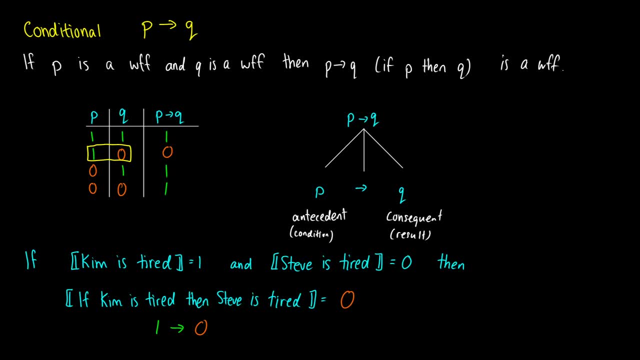 think about this as like the result, the condition and the result are the antecedent and the consequent. if the antecedent is met, then the consequent should follow from that. so that's the conditional. now you've learned all of the standard operations of propositional logic. sometimes there 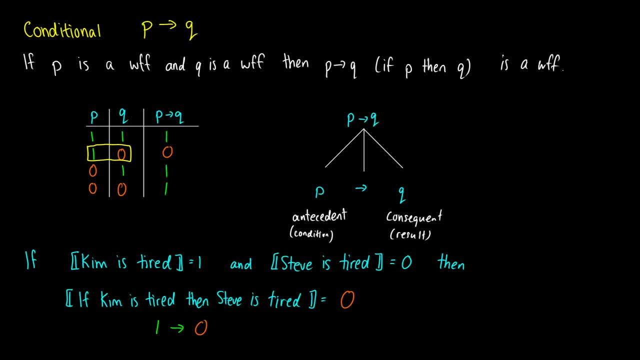 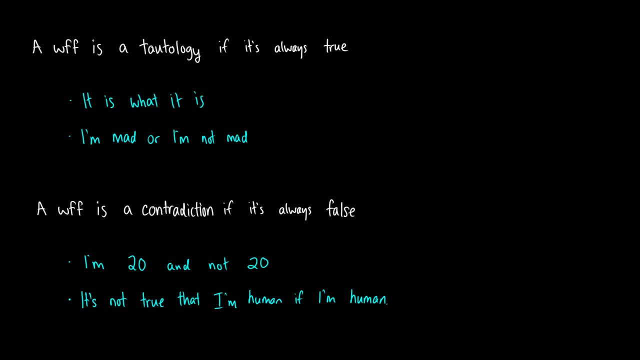 are other ones that can be used, but they're all combinations of the ones that you've just seen. in some way, the last thing we want to talk about are classifying well-formed formulas as tautologies or contradictions. so we have these terms called tautologies and contradictions, and a tautology is: 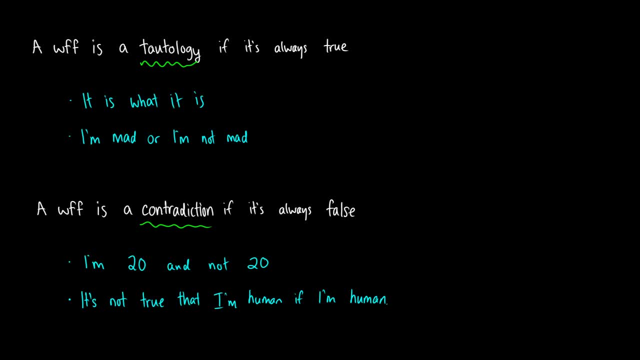 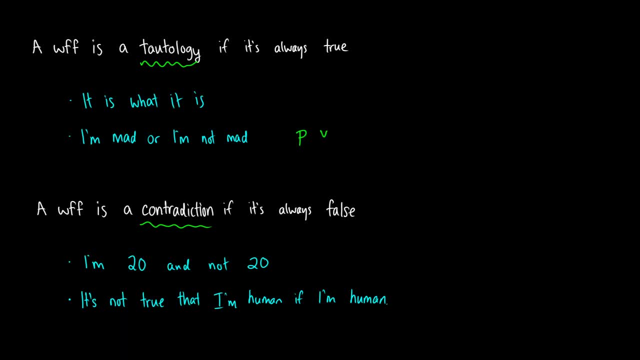